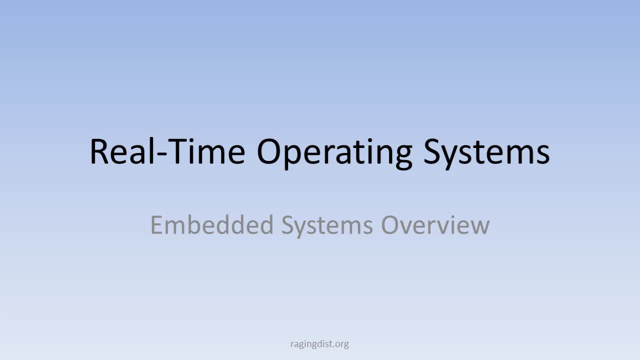 It's got everything documentation. it's got a make system. it's got a reference project that will run on an STMicro discovery board. It's ported to a couple different CPUs. It's got all kinds of features. It's great for beginners. It's also good for advanced users. 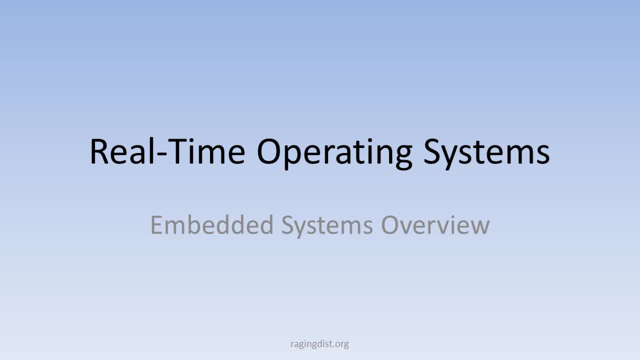 Now this first part in this series is an embedded systems overview. I'm going to go over terminology and general things about embedded systems and real-time systems. I'll then discuss how to set up properly for your aplications and how to build a real-time. 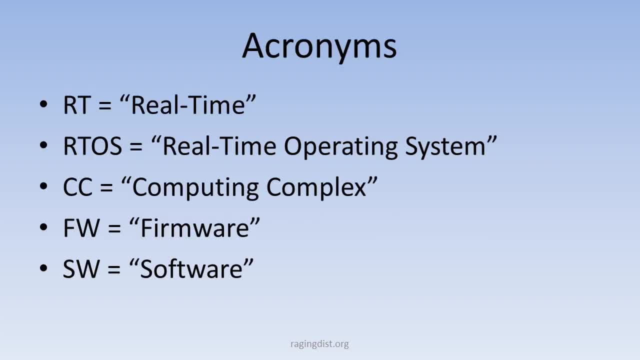 operating system. I'm going to start from scratch and I'm going to use my own acronyms. These things are used in the industry. They're found in text books. I modify some of these definitions to my own needs, to what I think they should be. I've added some of my own stuff, So the 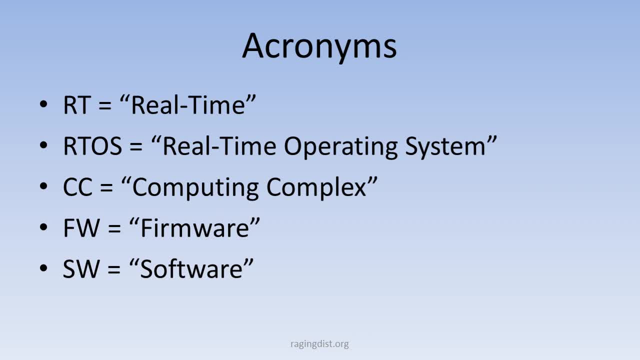 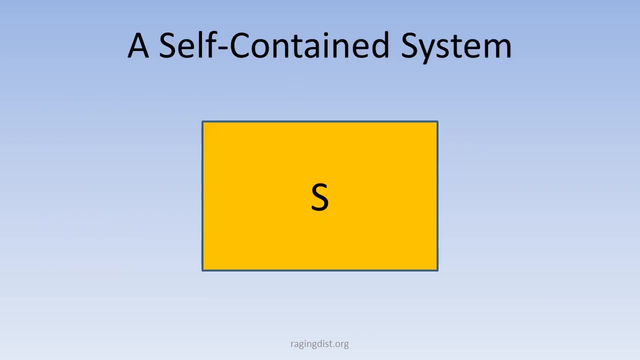 you're picky, i can't help you. these are the terms i've chosen to use here. i'm choosing to use them consistently, though, so bear with me if this isn't what you saw in a textbook, or this isn't what you use at your company, etc. etc. a system can be a self-contained system where it has a number of 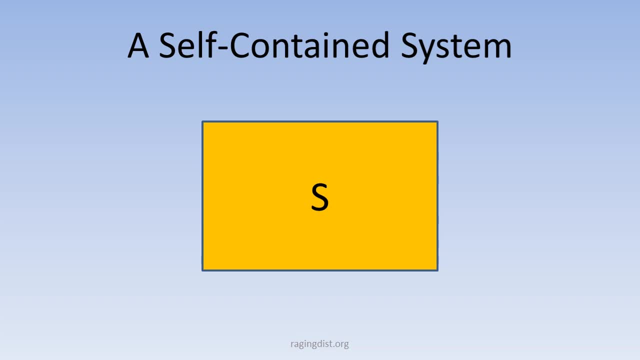 things that go on inside of it, and this system has no inputs and outputs inside of it can have several blocks. i'm not concerned about systems which are, which do not have the digital, and i'm going to use the word computers and and i'm going to violate terminology that i'm going 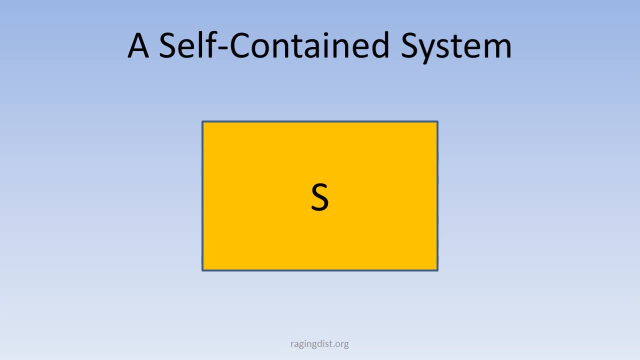 to explain later, but bear with me, and as i just used the word computer in an incorrect way. so a system is that i'm concerned about has some sort of a digital computer. there's different ways of doing that and there's different ways of fighting for that, and i'm not concerned about the. 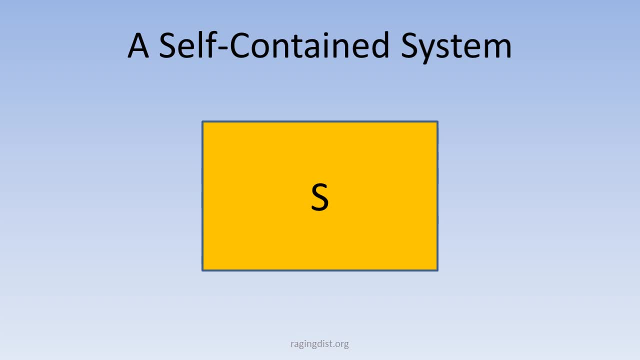 of making computers- and i'm not going to cover that- with analog computers, electromechanical devices, what have you? this system will have some sort of a computing complex and- and that's the the more exact term than computer- it'll have a computing complex which is a, for now, a digital. 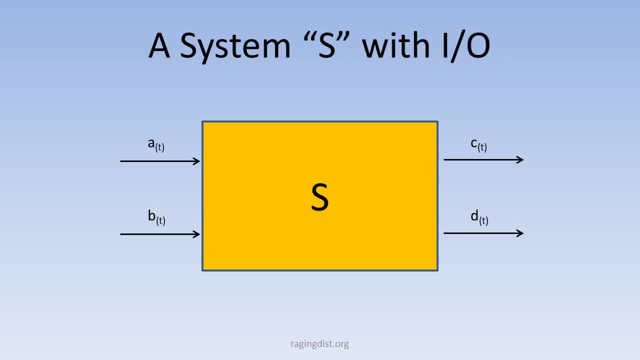 computer, never mind the other type of systems, the things you learn in thermodynamics, whatever. so the systems that we'll deal with can either have inputs and outputs going into the system, or the system can have all, can have blocks inside of it and have the inputs and outputs going on in. 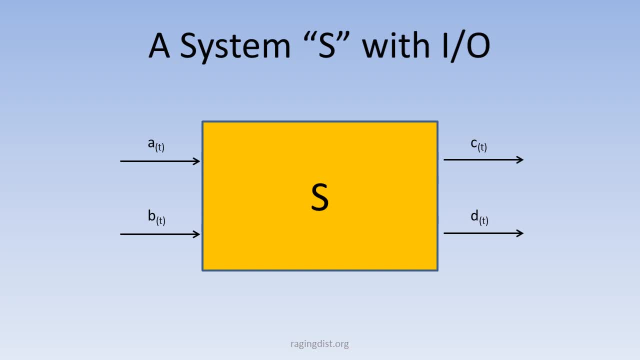 between sub blocks in it, but not through the boundaries of the system. it all depends where you want to draw the the line when you define what a system is. this could this diagram here. you could take this self-contained system in the previous slide, then just shrink the boundaries. 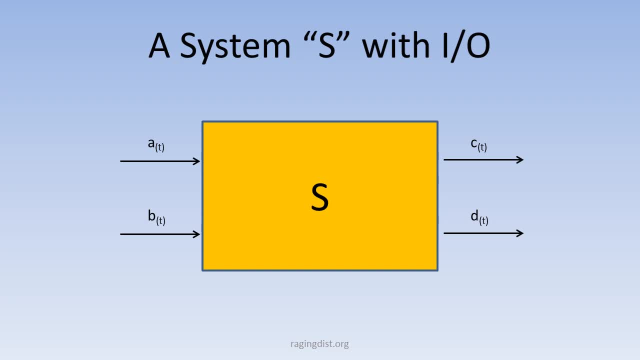 there and say that this sub block inside of the self-contained system is a system in and of itself and has inputs and outputs. but the point is you're going to have some systems which are self-contained, that you don't have inputs and outputs through the boundaries, and some which do. now they can. 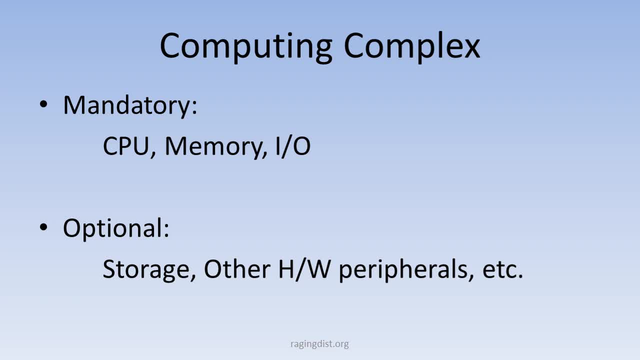 be connected with the properaku because they already have an input and output inside of it, but they're going to have some sub blocks in them that require inputs and outputs as well. so this is simple. it's not a big deal, since we know that this system is the only way that. 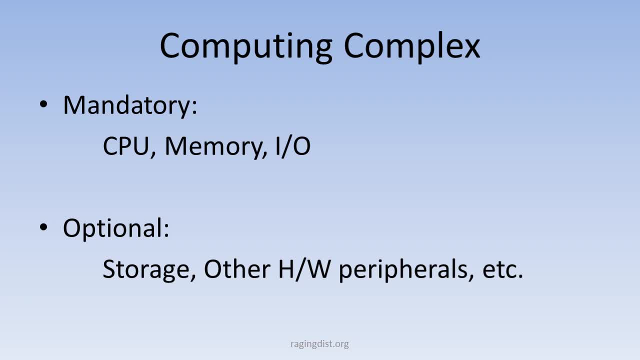 it's going to be in the system. so we now have a this that is a CPU memory, that's an i o, that's cpu. you can get into a lot of different things. i won't get into what it can be, but it be a system on a chip. but it will work with some memory, some ram memory, random access memory there. 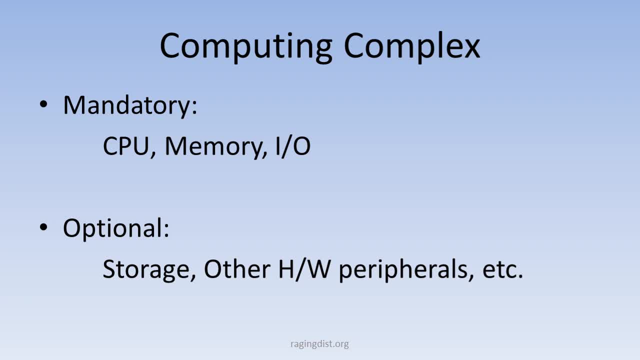 doesn't have to use ram, but i'm just going to call it ram memory, and the memory can also be flash memory, where you have a non-volatile type of memory. so you mix your volatiles, then your non-volatiles, and then it'll have some sort of io going into the computing complex. 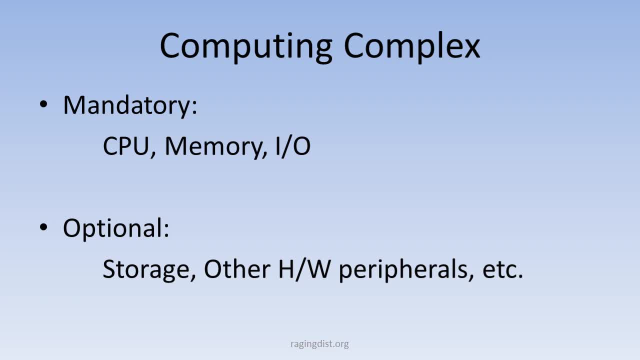 because what good is a computing complex if you can't access it right, these optional components which we're all familiar with: hard drives, any number of peripherals, on and on and on. these things are optional. you can have a computing complex which doesn't have these. most of them do. 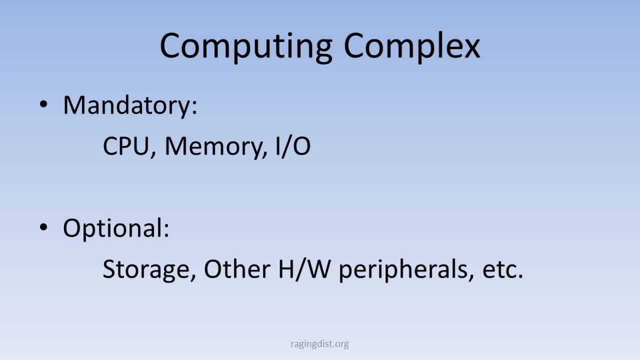 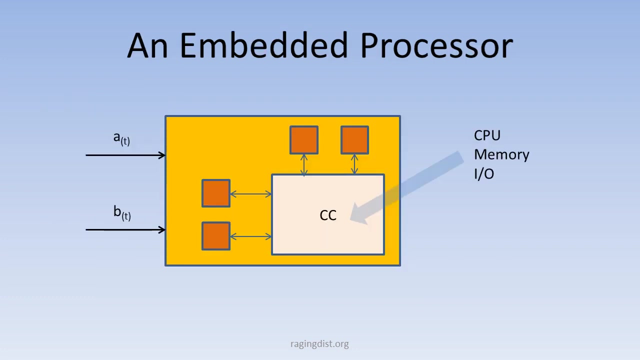 but i'm going to use the term computing complex throughout this presentation because saying cpu is not enough, saying computer is not enough, whatever, whatever other term besides that computing complex i think is intuitive just from what i put up here. now we need to discuss what an embedded processor is. 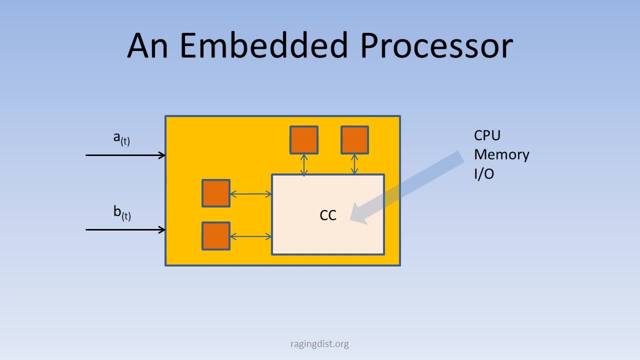 before going through all the other material, the you have used embedded processors- you've used them on a daily basis- might not have known that they're called embedded processors. an embedded processor will follow this diagram here and in this system. and this again, this is the yellow blocks with the system, which, in this case, the optional inputs, the. 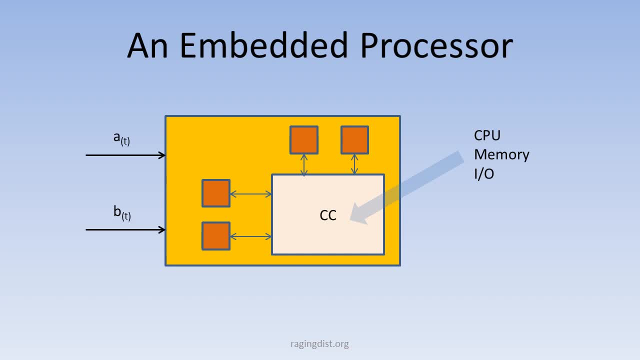 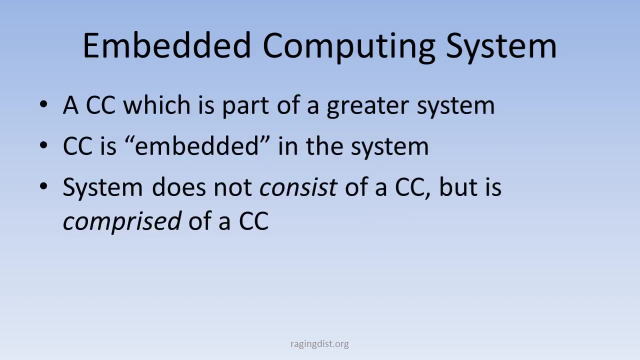 a sub t and b sub t, you can have a system that that's self-contained. the computing complex has other little boxes inside of the system that it talks to and the computing complex is thereby embedded in the system. the computing complex is part of of a greater system, like a car's braking system. the computing complex it is the cpu, the ram and the. 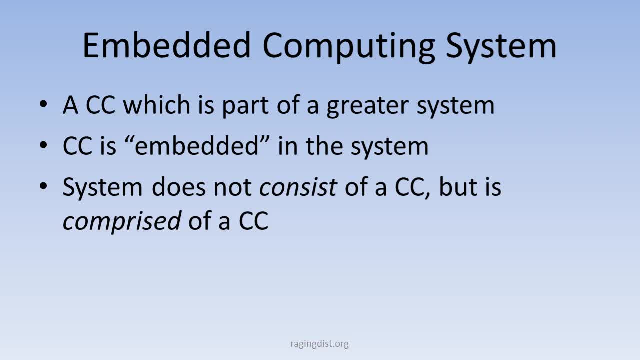 whatever, which then interfaces to solenoids, relays, what-have-you, and those things electromechanically will cause your hydraulic fluid to apply pressure to your calibers, to your drums and whatever that holds. that whole thing is your greater system, the braking system, computing complex, is one part of it. the 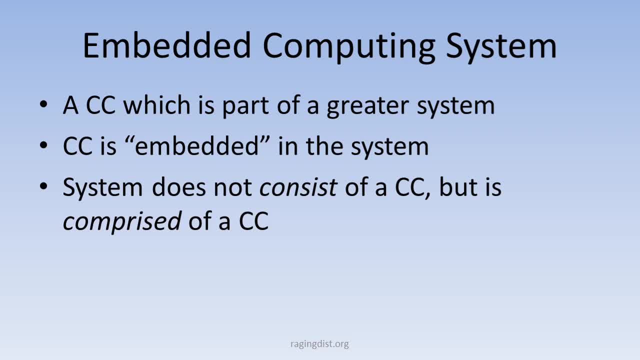 computing block complex is embedded in the system. it is. it is one part. it consists that the system does not consist of the computing complex, but is comprised of it. so the way you remember what an embedded computing system is is the word embed. you take a computing complex and you embed it into his system. 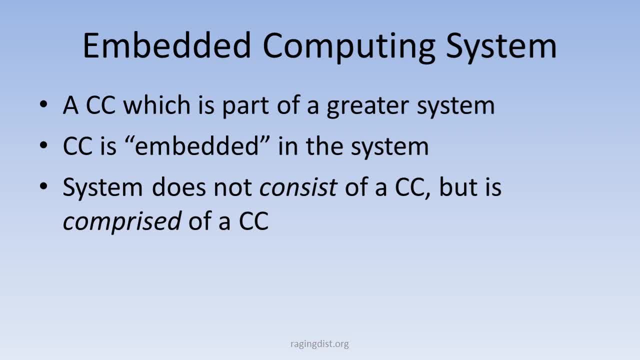 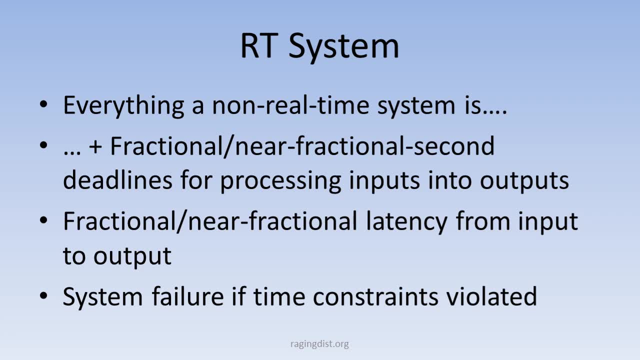 and that is an embedded computing system, real-time system- again, something that you've used. you use real time systems all the time and you've probably heard the term real time before. this has almost become like a slang word. you know, I need this done in real time. 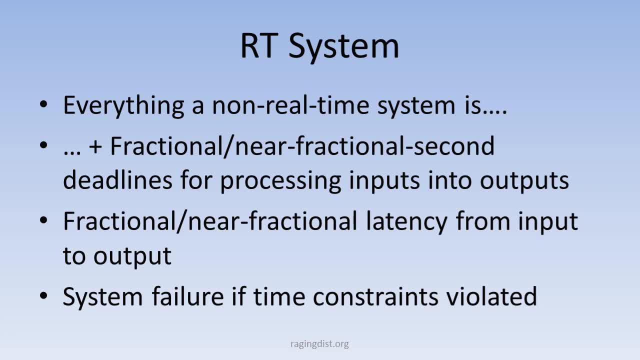 and through the usage of this term in slang, the definition has been lost to a lot of people that don't work with computers and the like. so a real time system is defined and the definition is not easy to nail down, even with people that work on these things and 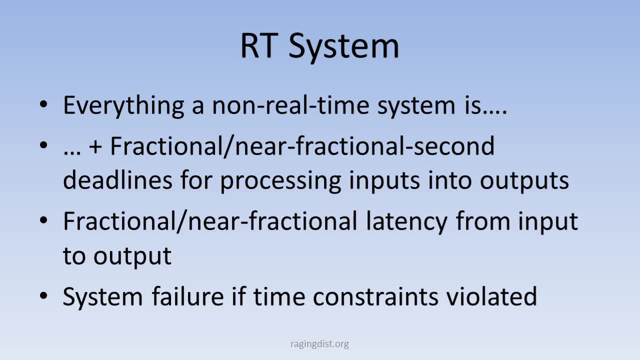 have written code and done testing and whatever for years. if you were to corner them and say, define for me what a real time system is, they'd probably have a difficult time doing this. I stumbled across this definition in a book once and this is my best definition. 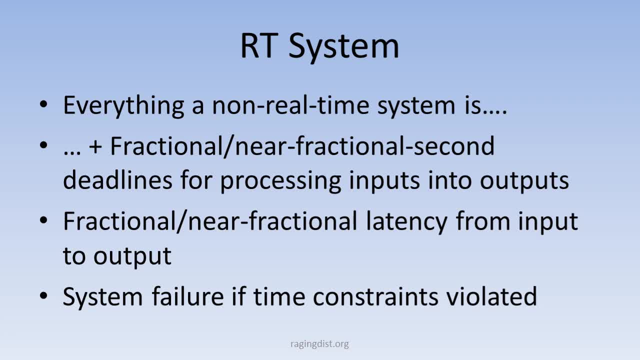 so before I define what a real time system is, first take an ordinary computing complex, whether it's embedded or not, and that computing complex, that system, the non real time system, must work according to certain rules in a digital system. in a computer, there are timing constraints between the CPU and RAM. 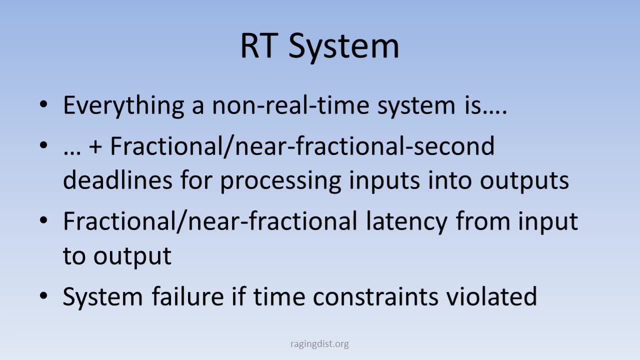 which run down into the nanosecond, picosecond range very tight. if you overrun some of the timing there, then the system will will crash. the hardware isn't working correctly. that does not make it a real time system, even though there are timing constraints built down inside of the computing complex. 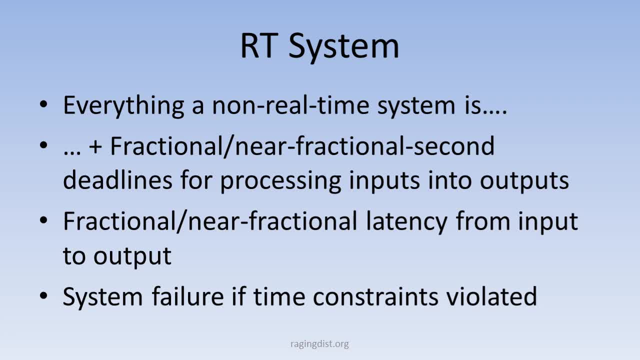 those things are contained in the computing complex, but that is not a real time system. but my point is is that any type of computing complex has lots of rules. it is a machine which there are contracts between the internal parts of the machine which are any of them are violated. 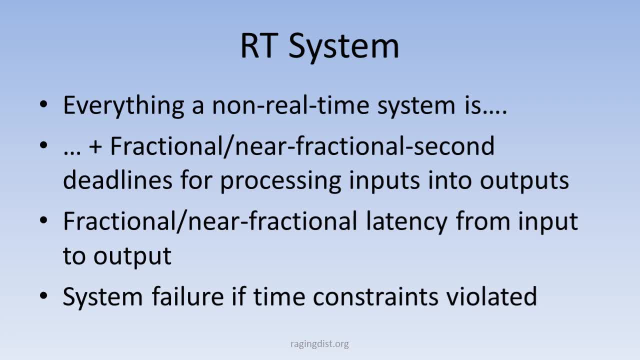 will cause a failure. so so let's bring this over to a real time system now. a real time system, first of all, must do everything that a non real time system does. so the non real time system has timing between the CPU and RAM, the real time system inside the computing complex. 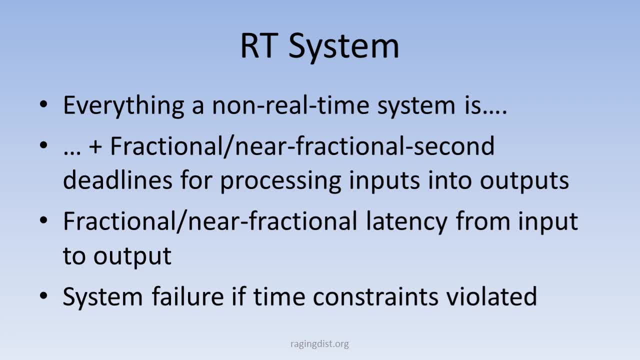 also has timing constraints. real time systems can use computing complexes that a non real time system does. so the real time system, at a minimum, has to do everything that the non-real-time system does. It has to follow all the rules, It has to execute code, etc. etc. 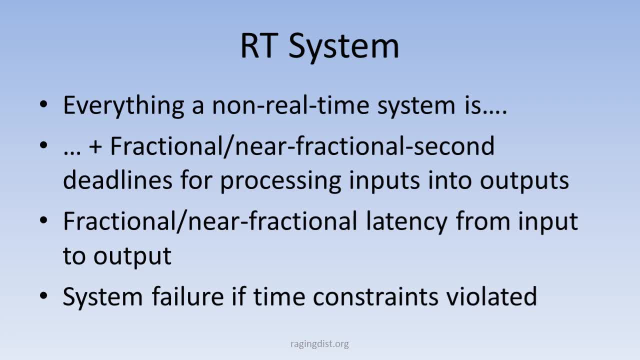 What makes a real-time system different than a non-real-time system? It must comply with timing deadlines as part of the system. The system itself has timing deadlines, either in the sub-blocks inside of the self-contained system or on the IO coming in and out of the non-self-contained system, one which has IO. 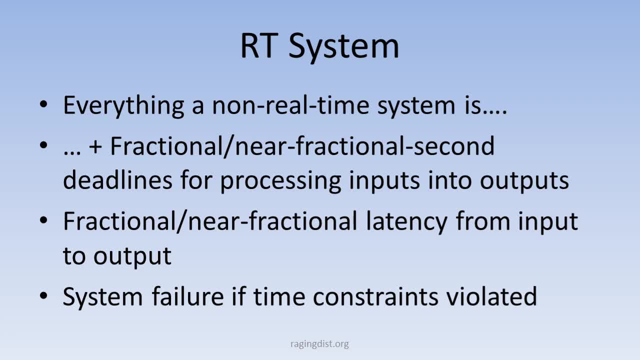 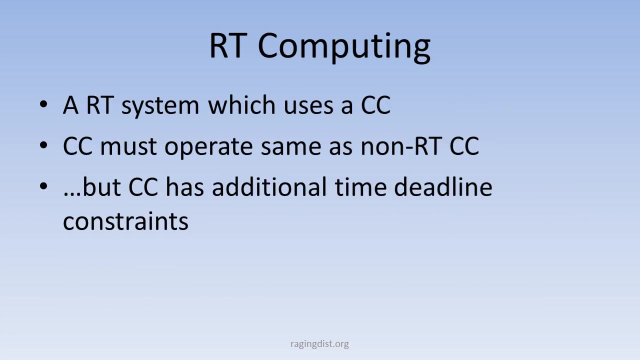 These things must be done according to whoever specified the system. The timing must be obeyed, Otherwise you have a system failure if these timing constraints are not met. And this gets complicated because the timing constraints are not necessarily a hard wall. So to review a real-time system is a system, the real-time system that I'm talking about. 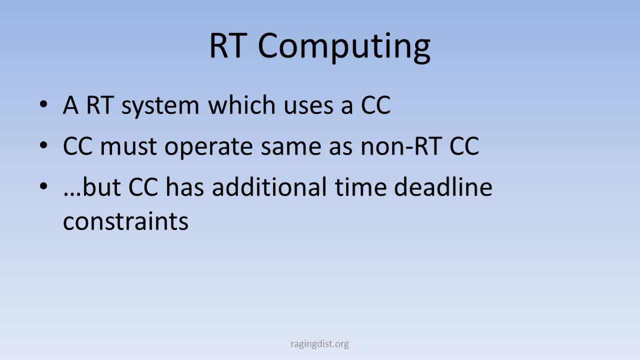 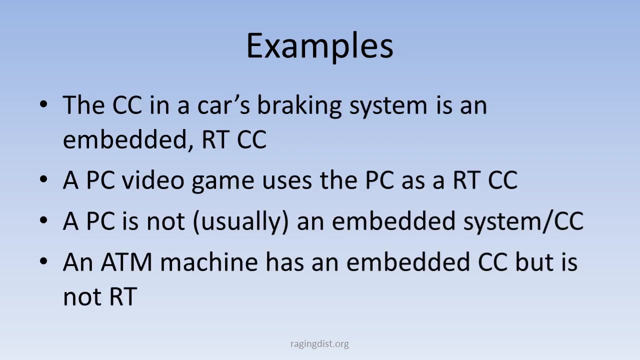 because people have made real-time systems in the past which don't use computing complexes And, as I said at the beginning, I'm only concerned in all this, in digital computing complexes. but a real-time system does not have to use that And the real-time system must operate the same as a non-real-time and meet the deadlines. 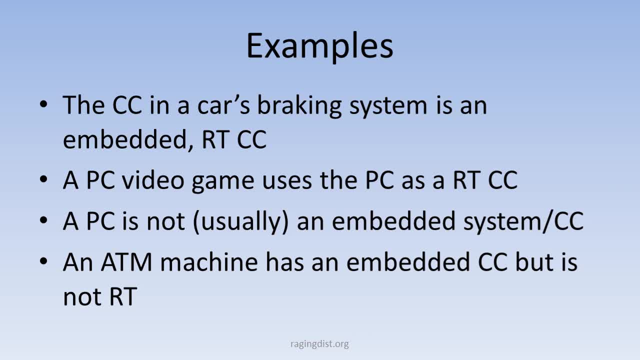 The examples that I've said before, and some of which I'll add here, are things that we've used in our day-to-day life. The computing complex in a car's braking system is an embedded real-time computing complex. As I talked through this before, the braking system is an embedded computing application. 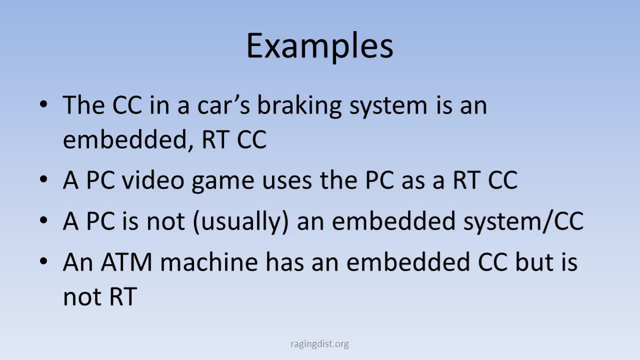 It has an embedded computing complex, but it is, in addition to being embedded, it is also real-time. You're going down a hill. You don't want your car's braking system to delay processing. So an example of a non-real-time system is a download of a file from the Internet. 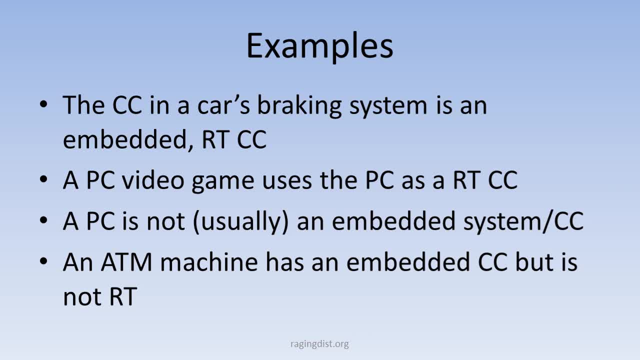 A download of a file from the Internet can be kind of choppy. You can have the thing down. you know the file can come from some server and it can download a whole bunch. So you can have the first two seconds of a 10-second download and then just pause for five seconds and then get the rest in the last three seconds. 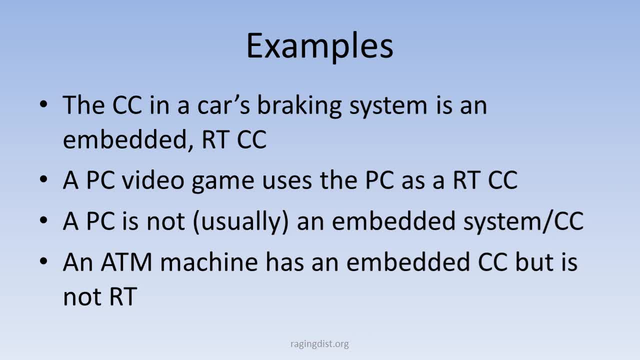 That's okay in a non-real-time application like a file download. In the case of a braking system, you cannot have the brakes, just not do anything for two seconds and then play catch-up like in a file download. That violates the real-time constraints. 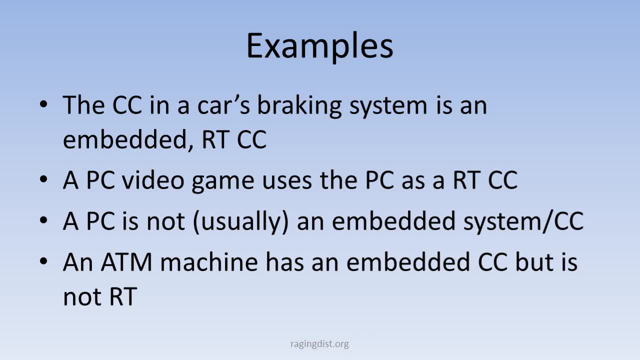 That braking system is is is a failure of a system. if it does that- and the next example is a pc video game. pc video game- you will use a pc. a pc is not usually not, because sometimes a pc can be an embedded system. if the pc is being used, let's say at the dentist office, to run some of their 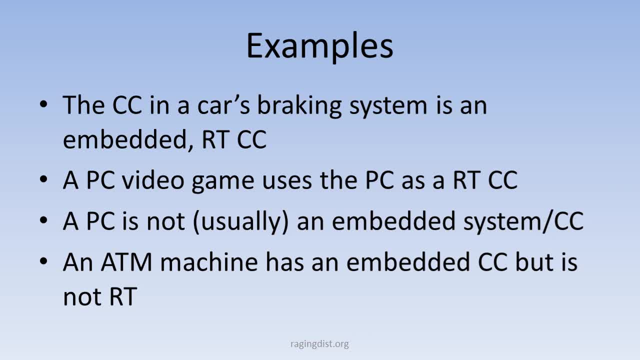 equipment, but normally a pc is not an embedded computing complex. the pc video game, however, is an application which uses that non-embedded computing complex to run a real-time application, the game. so the computing here can be embedded, the computing can be real-time, it can be. 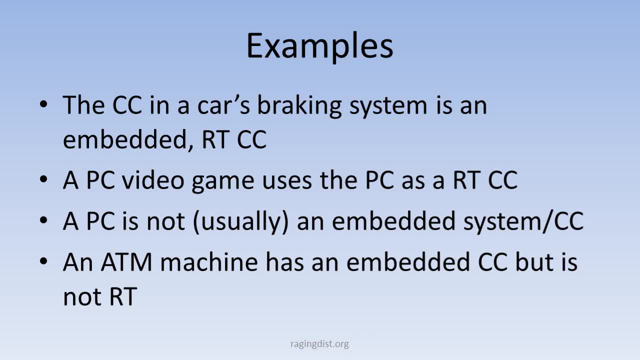 one. it can be one of either embedded or real-time, or it can be both. embedded in real-time, it's it's depends on this system. so an atm machine is another example it's it's. it has an embedded computing complex, but there's a part of it. there's a tiny part of it, the keypad which 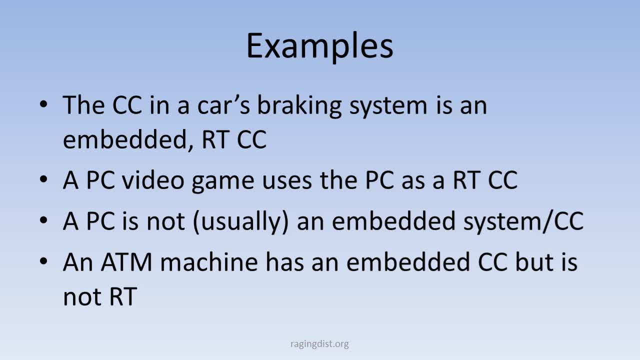 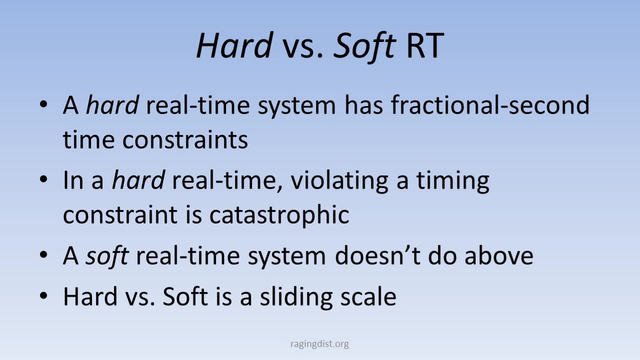 is real-time- and i'll give another example similar to that later. but generally speaking, the atm machine is not real-time, though it is embedded. there is hard real-time and soft real-time and real-time. one of the reasons why real-time is difficult to define is because this- uh, the deadlines that you overrun- can be hard. 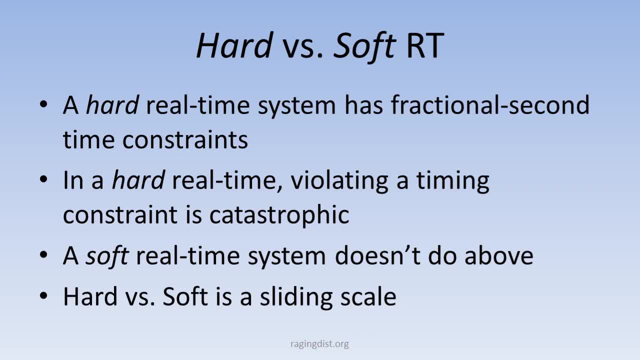 deadlines, and they can be soft deadlines. it all depends on the nature of the application. a hard real-time system usually has deadlines, timing deadlines, which are in the fractional second range, although that fractional second range can vary depending on the application. so so the the video game example, the fractional 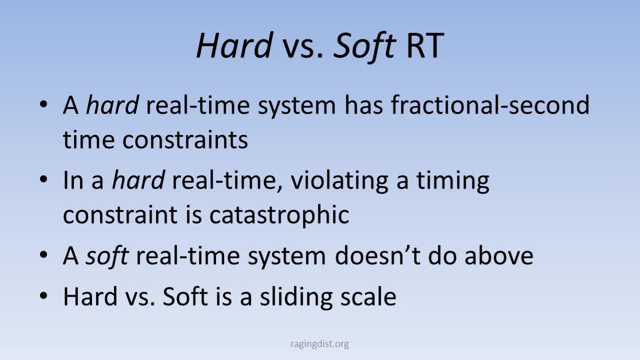 second, deadlines are in the hundreds, anywhere from, say, 100 milliseconds, 10 times a second, down to a hundred times a second, 10 milliseconds. but if you jump over to an application of a servo controller for a motor controller, that thing can have hard time. deadlines below 10: 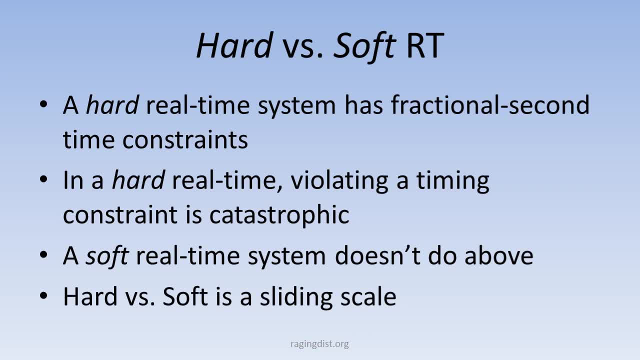 milliseconds, usually below 10 milliseconds, even below one microsecond. where a violation of that of that computing? if you have a system design where every one millisecond a motor control system say, well, let's just say it's 200 microseconds, you have to read where the position of the motor. 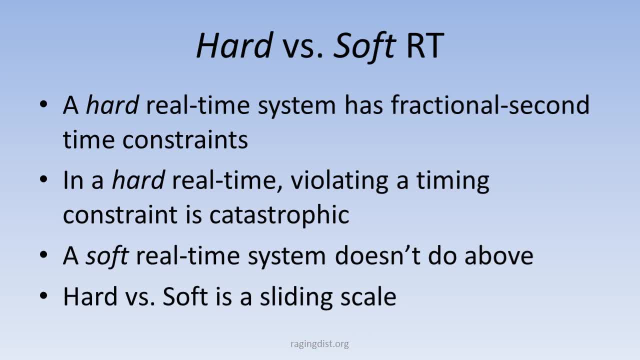 rotor is, and then the 200 microsecond time frame and then compute a new drive for it at the end of that 200 microsecond frame. That is hard real time, because if you do not, if you set up your frames to operate every 200, 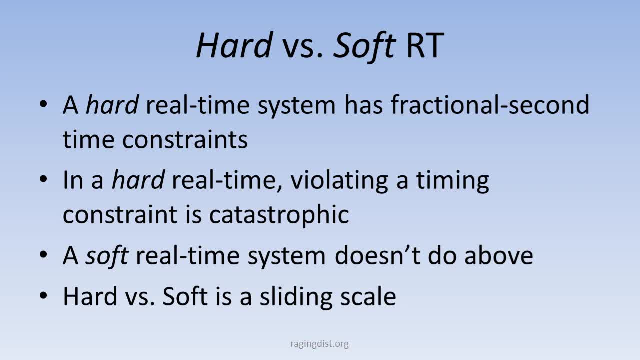 microseconds and you don't finish your computation at the end of 200 microseconds, you are in a state of failure. In a motor control application like that, you would expect the system to shut itself down because- because it's not designed to fail like that, It's got safeties in that to detect it. 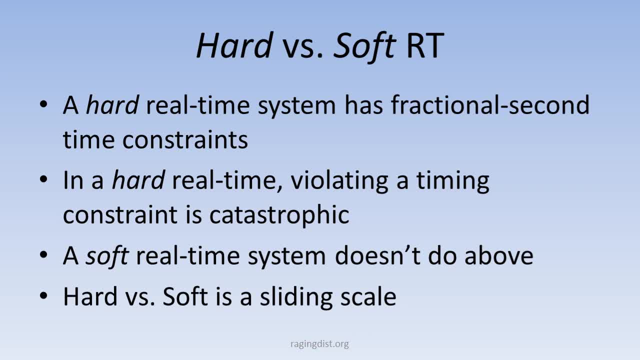 and there's it could. it could cause a loss of life, damage, whatever. So the system has to shut itself down, maybe restart or whatever, because it's not working correctly. A soft real time system: that doesn't have to. you have a. 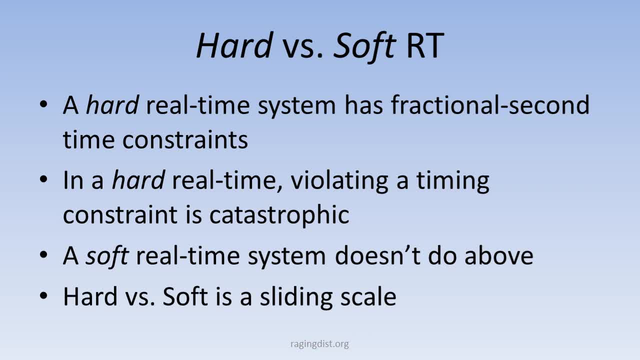 violation of the timing. it doesn't have to set its to shut itself down that the timing violation can be a nuisance violation, but it's one where the system will continue to work. It's continued to work in a way that wasn't intended to, but there's some. 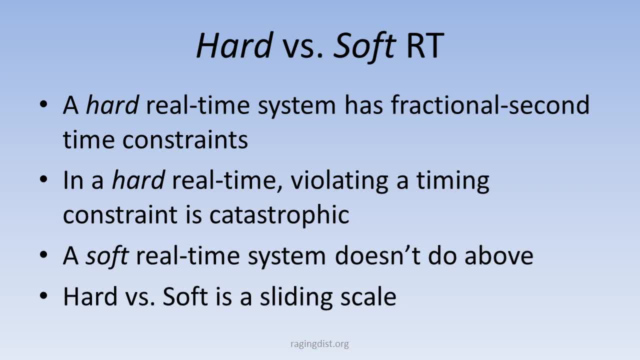 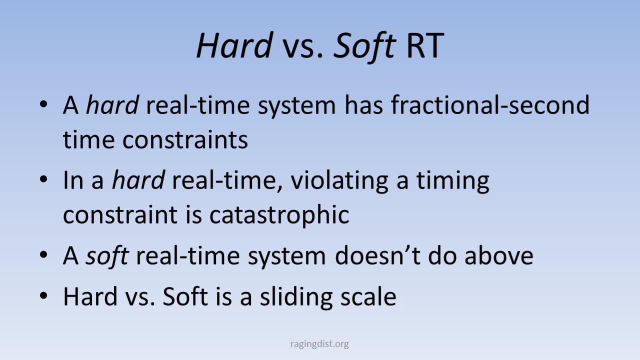 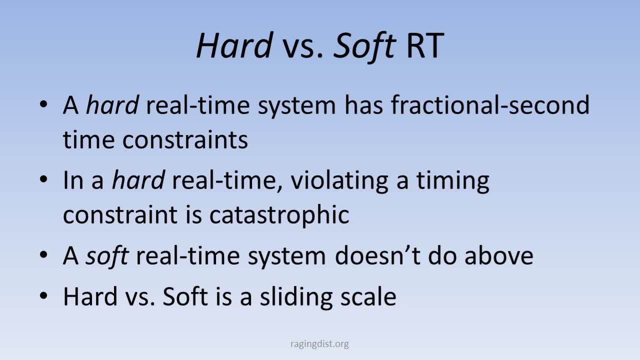 The system seized up and you hit the number five but it didn't take it. And you wait three seconds and you go on and you realize it didn't take the number five because it was seized up or something like that. That's a soft real time example, Annoying. but the system is not in it's, it's, it's. 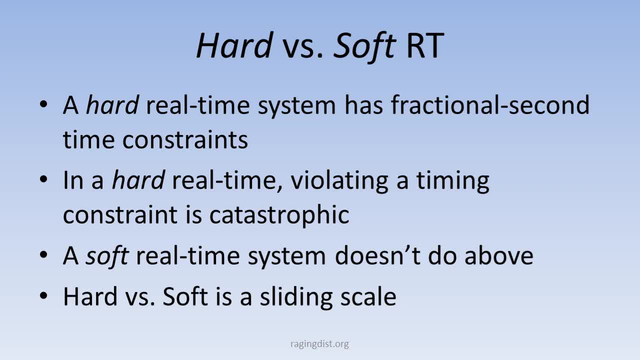 it's not a catastrophic failure where it's not in a state where it has to be shut down like the motor controller. So this, so this hard and soft real time stuff is it's all a function of what the system is set up to do. It's like I said, there's no hard boundary. It you, you can have. 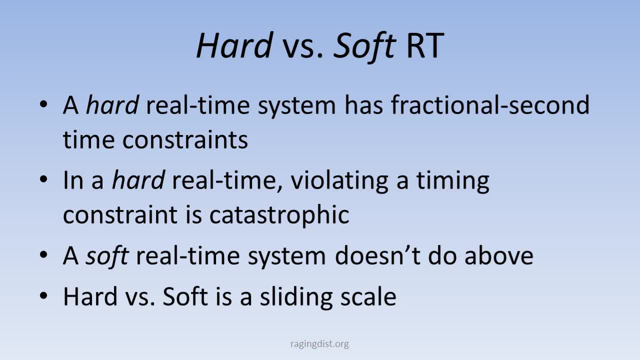 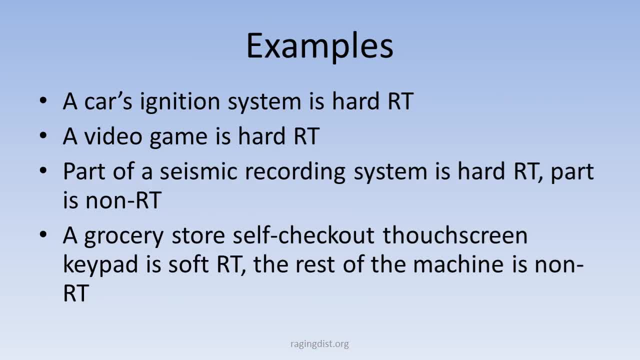 it's hard real time. Some more examples here of these hard real time, soft real time. Car's ignition system is hard real time. Ignition system is, of course, when you have to determine when the spark plugs actually fire, based on how the the, the position of the cylinder heads and 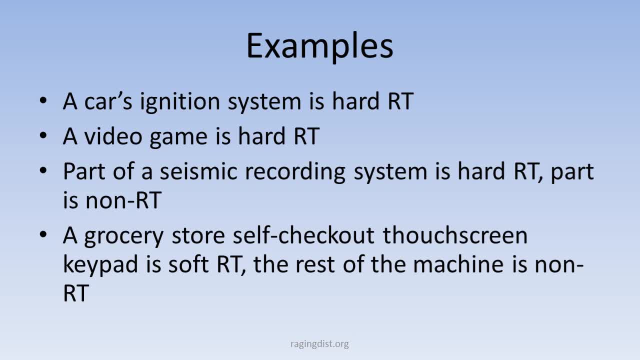 a number of other calculations that your cars embedded computing complex- And notice I didn't say the word computer and most people would- but the car's embedded computing complex must calculate when precisely that spark has to go out to the spark plug. If it's off by a large amount you could get a bad knock in the engine. 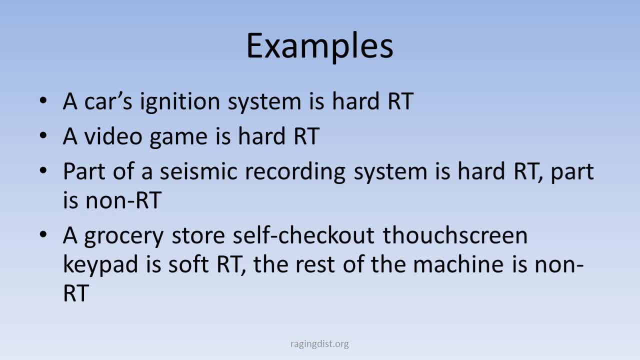 and that knock, if you get too many knocks or if you get a severe enough knock, you could end up damaging the engine. Video game, as I've said, is hard real time. Now, a seismic recording system is partly hard real time and partly non-real time. So seismic recording system and it could be- 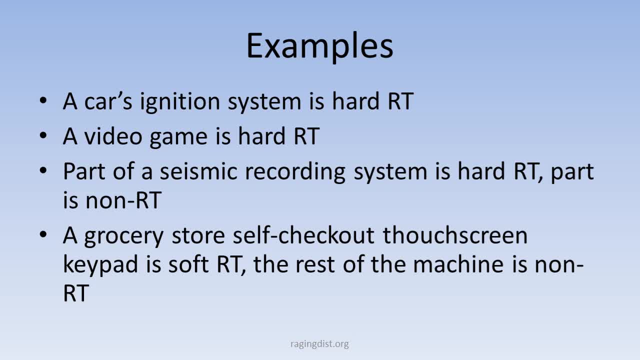 and then let's just say it's the. you've got a mountain range in California that's prone to earthquakes and every hundred meters that you put these sensors into the ground to measure the vibrations in the ground, and then every 10 milliseconds, 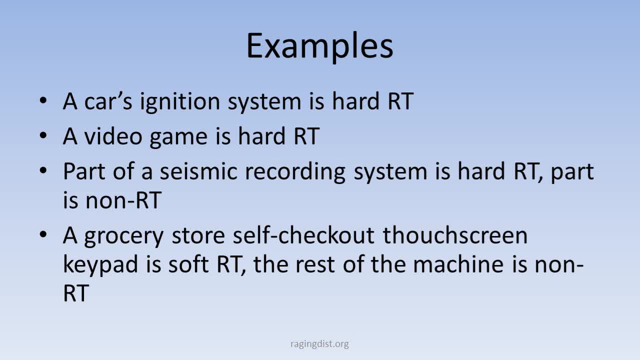 I'm completely making these numbers up. They could be in the order of seconds for all I know, but let's just say every 10 milliseconds you record the, the vibrations in the ground. put that into an analog and digital converter and that conversion. 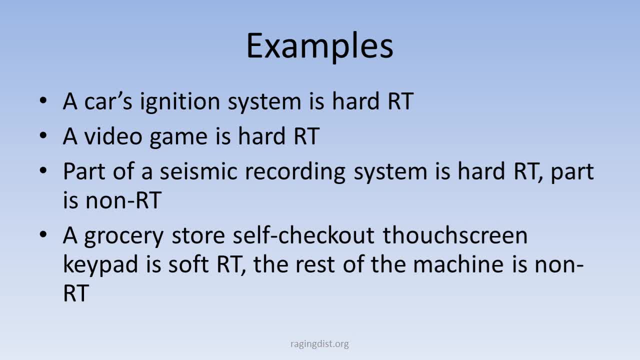 gets stored ultimately gets stored in a database somewhere. So you have to have a precise measurement of the ground vibration every 10 milliseconds. But once the data is stored into a database, you could have somebody at a office in Los Angeles who is reading this data back. 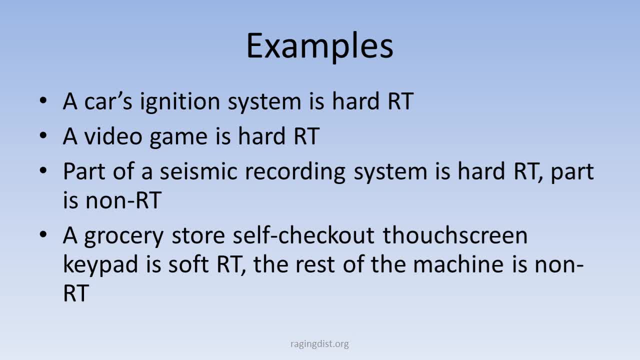 that's been put in databases and that whole part of the seismic recording system, where that data is in the databases, is not real time. The data is just buffered up and recorded in hard real time but the rest of the system does not have to run in real time. And again, the grocery store. 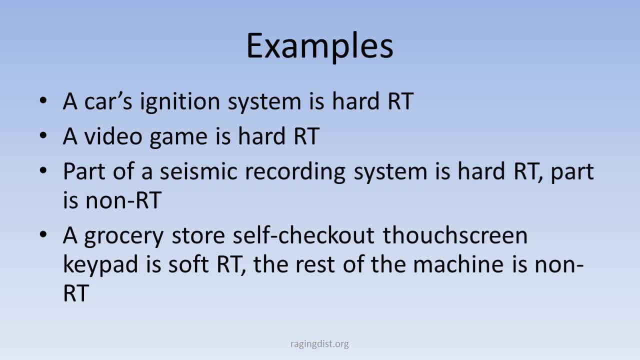 self-checkout touchscreen is soft real time. The rest of the machine is not real time. So you can, you have a soft real time component like the touchscreen and you can operate with something that the user- the user punching in numbers, the user expects when he or she comes around to being prompted to enter the type of payment. 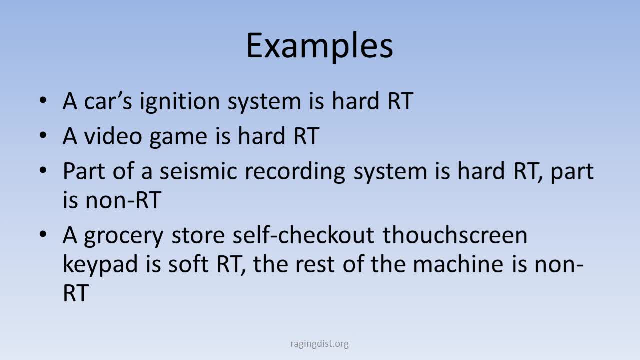 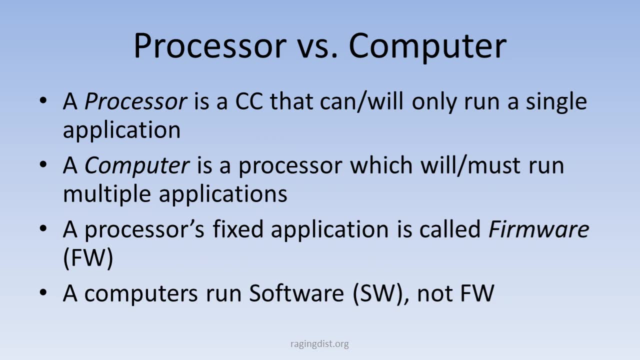 or something that there will be a variable delay But the user will not expect there to be a delay when entering numbers. So you've got the soft real time working with the rest of the system which is non real time And- and there are more examples of of this- the fluidness of this, of the real timing aspects. 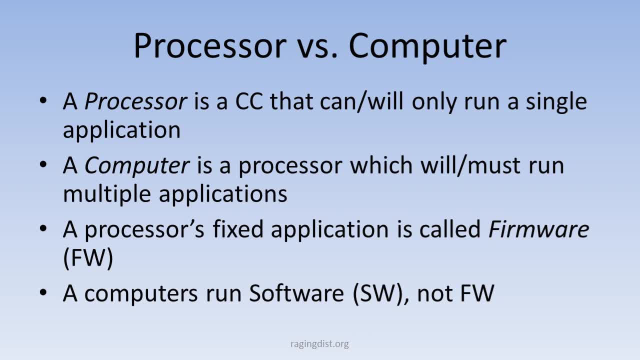 Processor versus computer. We normally use the word computer, as I've said before, to mean everything that, that, that that I use the term computing complex for You have a computer in your car. You can actually have many computers in your car. You can actually have a computer in your car. 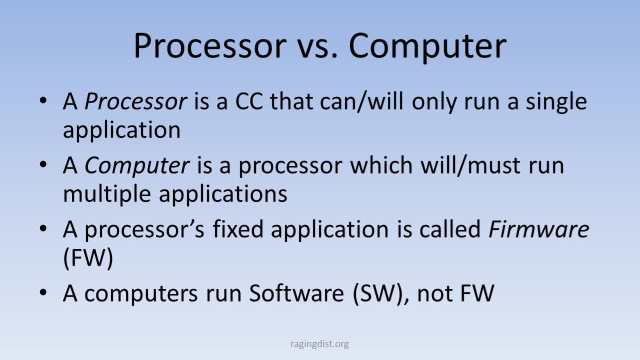 But you ask the average person walking down the street describe a car nowadays? Does it? and they'll. if they have any knowledge of auto, of an automobile, they'll say: and it has a little computer in it and that computer runs the engine Technically speaking, according to the definitions, that 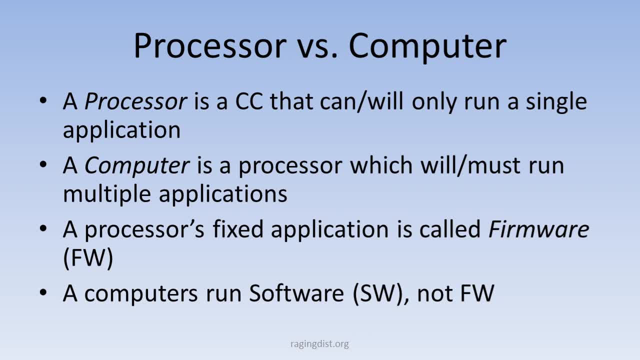 that, that that are in this presentation and what's in textbooks, what's in the industry? when you drill down to this definition, that computer in your car is not a computer. the computing complex is is actually a processor and not a computer- A processor by definition. 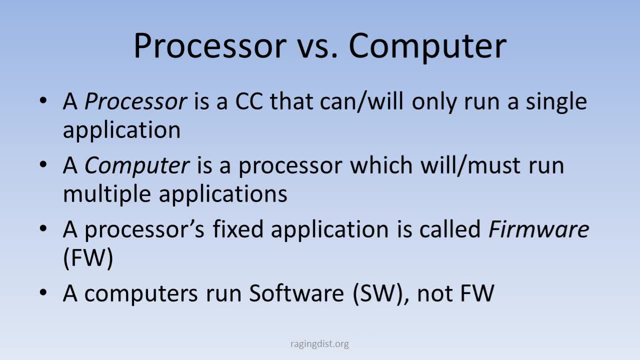 will only run a single application. Computer, by definition, is a processor which is designed to which will, which, which must run multiple applications, The. this is why ENIAC is considered to be the first computer. actually, Let me, for the record, say that recently ENIAC has lost their place. 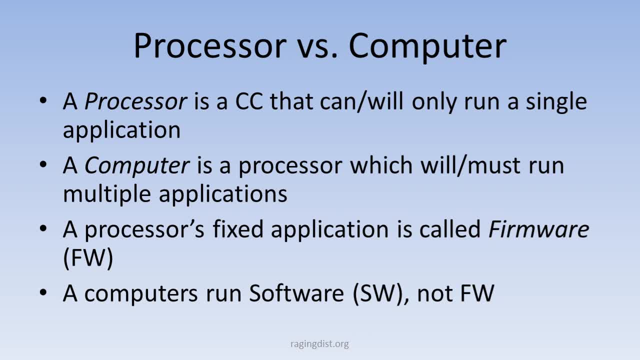 in in the the annals of computer science history. It is not considered the first computer anymore, but I'm going to use ENIAC as an example of the first computer. It was the first time that they were able to have a machine, a computing complex, which they could change out. the 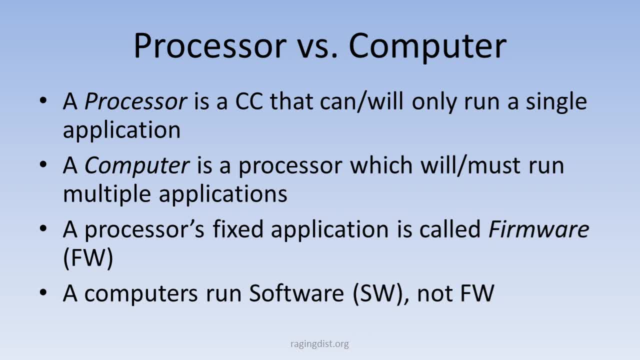 application which it ran, Change out- with difficulty of course, but still change it out- The processor that that can just run one application. and then they were probably processors. before ENIAC, the processors did not qualify as being computers because they. 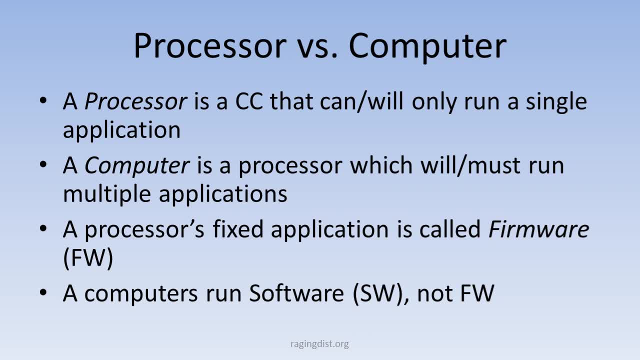 had the fixed application, so the, so any processor before ENIAC was made. Indeed, it didn't qualify as being a computer, so it's not enshrined in the Smithsonian as such A processor, since it only runs one application. that processor's fixed application we will call firmware. 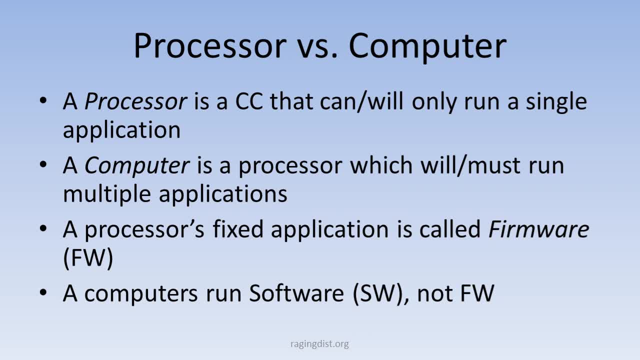 Firm, meaning that it's not going to change. It's not intended to change, It's going to just run the one application. That firmware can can be in flash, it can be on a hard drive, it can be in any type of memory, but it's not like the software that a computer runs. 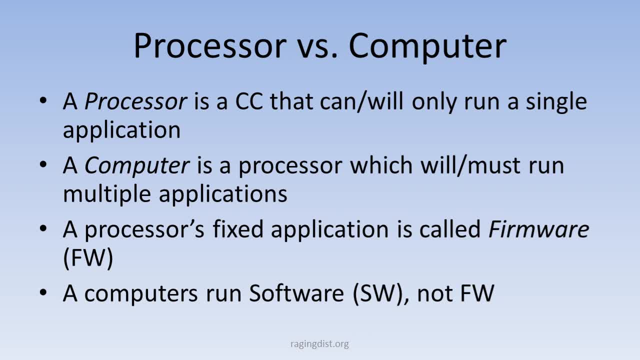 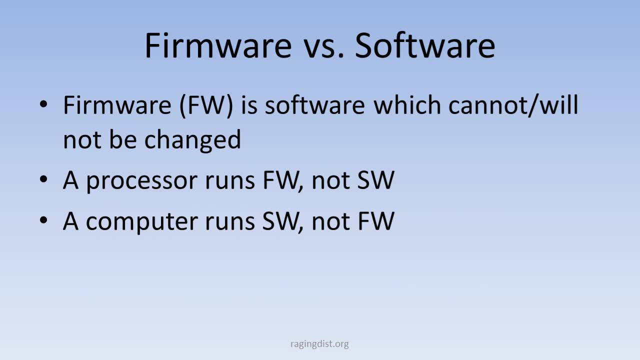 Software is the applications which can be changed in and out that run on a computer Processor running firmware. Firmware can be the same processor. I mean I'm sorry that the computing complex which runs firmware, The computing complex running firmware, can be the same computing complex in firmware and a processor which is used in a computer running software. 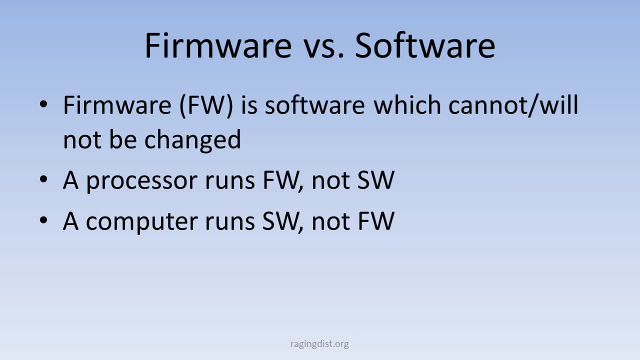 So there's no restrictions on what type of computing complex It can be put inside of a processor-based system or a computer-based system. The one can run firmware, the other can run software. they can actually both run on the same type of storage medium. It's just that the intention of the software one is to change that. 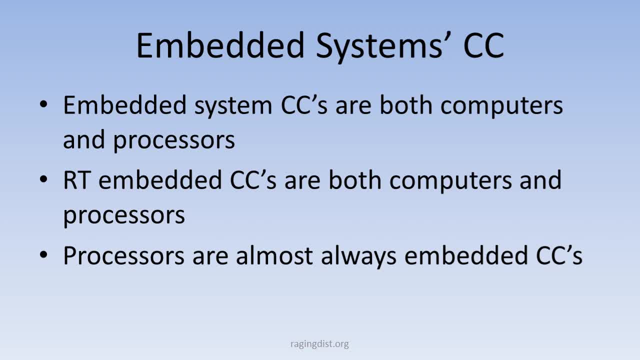 So embedded systems having computing complexes can be both computers and processors. Usually, an embedded system is going to be a processor, but there are embedded systems which run computers instead of processors. This gets more complex and I won't get into it. I'll let you stop and think about. 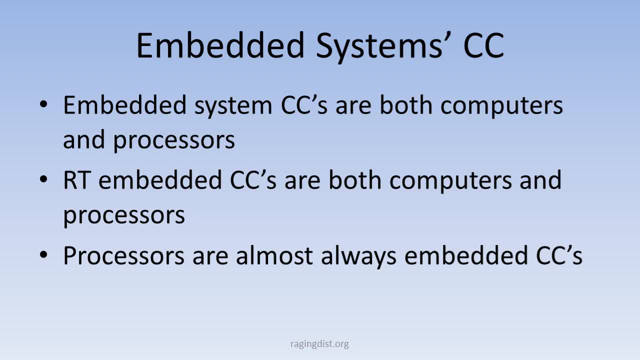 when you would use a computer in an embedded system. Real-time embedded computing complexes are both can be both computers and processors- again just like an embedded system, and you're seeing a lot of overlap here. Usually, though, let's say usually in the video game example, it violates that the usually function doesn't work here. 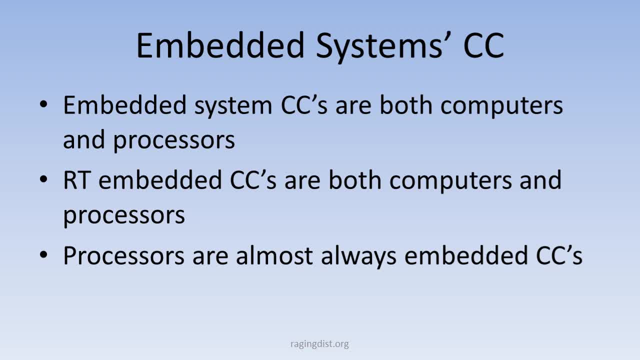 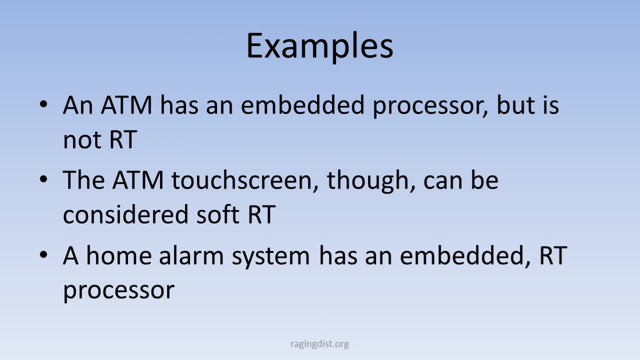 the usually for a real-time non-embedded system, but usually for a real-time embedded computing complex. again like the non-real-time embedded computing complex, you're going to use a processor atm machine. it has an embedded processor, not real-time atm touchscreen like the grocery store touchscreen. it is another soft real-time example. home alarm system has an. 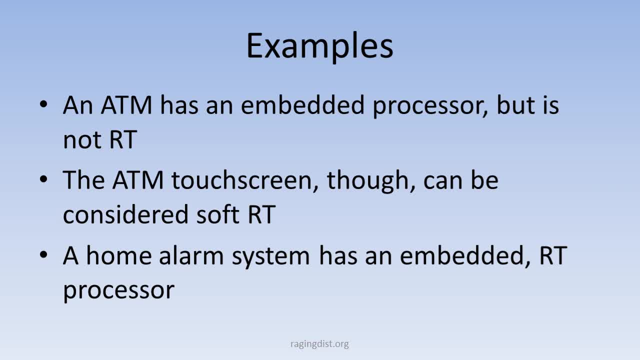 embedded real-time processor. you can make a home alarm system on a computer. you can use a. you can use a PC which is a computer for a home alarm system. it is embedded because the system's got sensors. it has a window opening detectors, motion sensors. it's in real-time, soft real-time, you could argue. 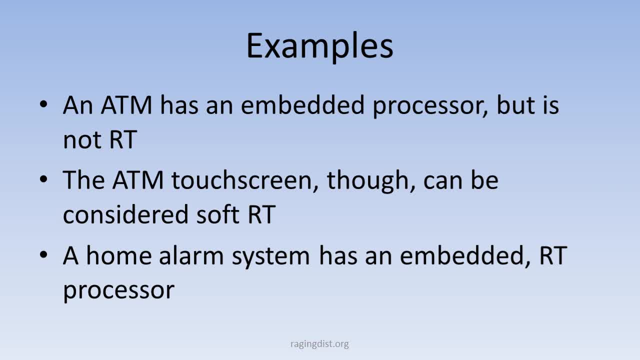 but the system is in real-time. usually it's, it's, it's. it is a process. it's a little standalone unit that you buy which only runs the home alarm system. but, like I said, it's an example of a computer: computer, uh, uh, will enter the isolation again to create a home alarm system. 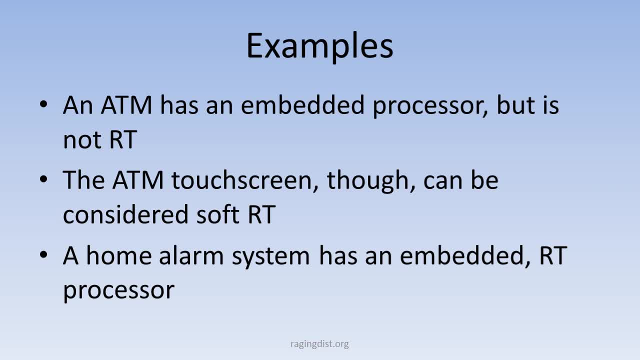 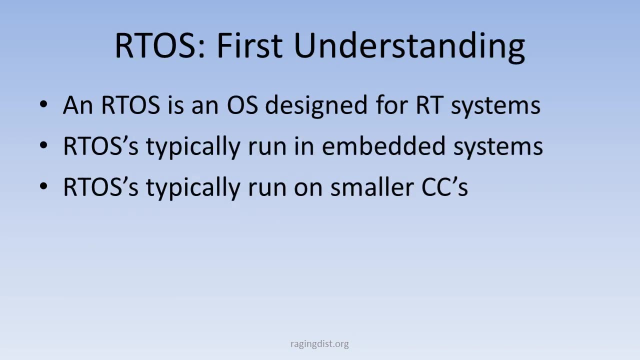 well, thank you guys for staying, and I'm sure you'd be better off with a processor, cuz your computer can't always act as the alarm system if you're, if you're rebooting it or getting a Windows upgrade or something like that, but you get the picture. 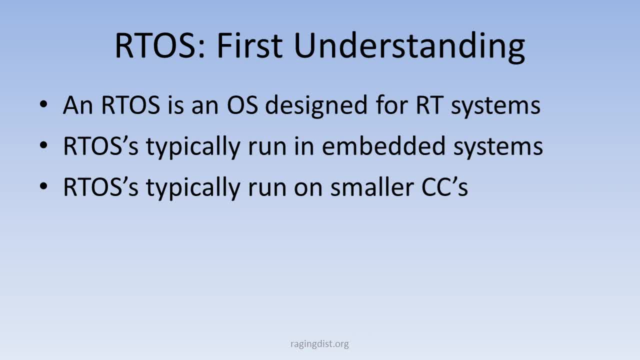 so this company, to the end of this long presentation about the differences, the subtle differences, between embedded systems, non-embedded systems, all this was done. the real-time systems, etc. etc. all this is done to give you a first understanding of what an RTOS is: real-time operating system. 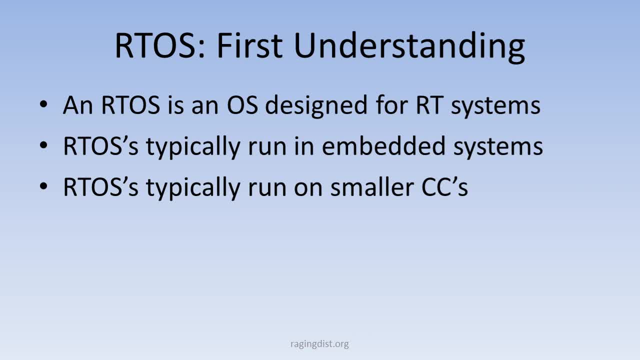 Without understanding all these concepts which I said before, you cannot begin to understand what an RTOS is. What is an RTOS? as a starting definition, An RTOS is an operating system designed for real-time systems, real-time systems, of course, being ones which use computing complexes. 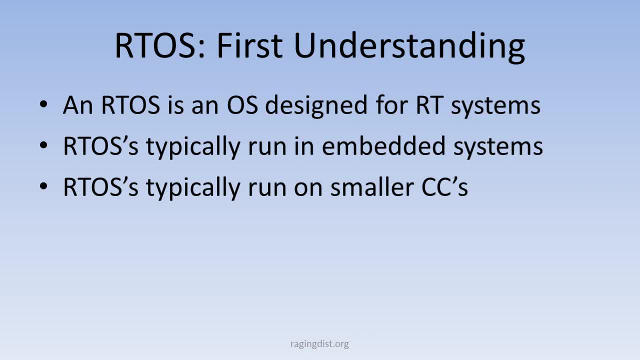 RTOS is typically. RTOS is typically a system designed for real-time systems. They run in embedded systems but they don't have to be embedded. It's not a constraint for an RTOS, but you usually find that RTOSes. 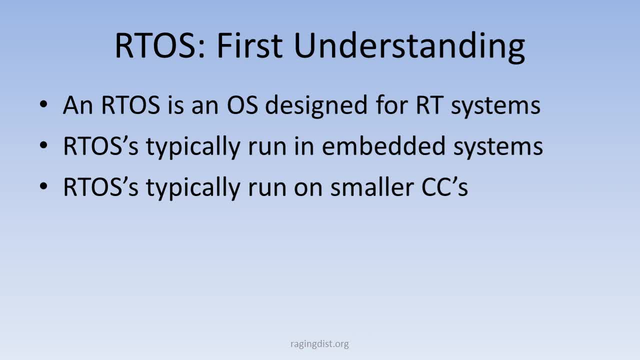 as we use in the industry, usually imply a certain type of operating system. So an RTOS has a couple of definitions And these definitions aren't always the same. It depends on the context When you talk about an RTOS. it depends on the context of the conversation. 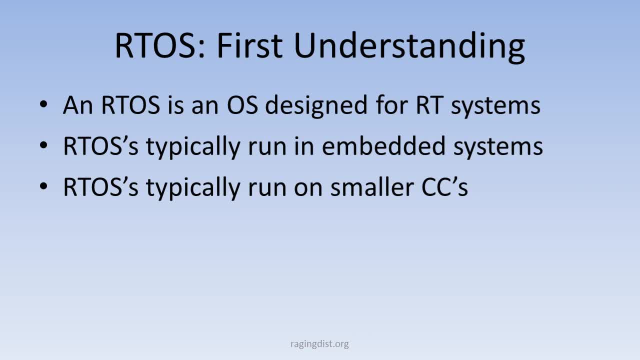 which definition of an RTOS you're using. So the first definition here: an RTOS is an OS designed for a real-time system. You can design an RTOS and they have designed RTOSes if you have an Aegis. 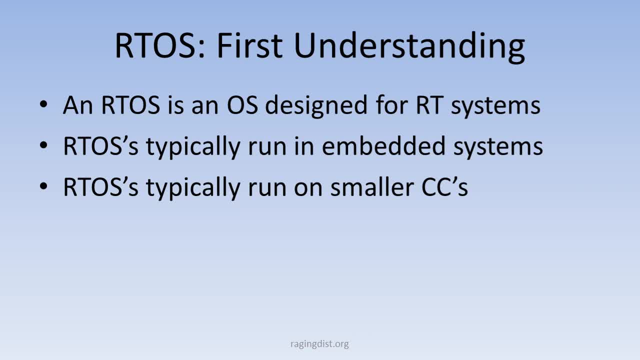 If you have a cruiser, a Navy ship has a real-time operating system which runs all of their missile control, their fire control systems in real-time. But this last definition here I've got as an RTOS, typically being something running on a smaller computing complex. 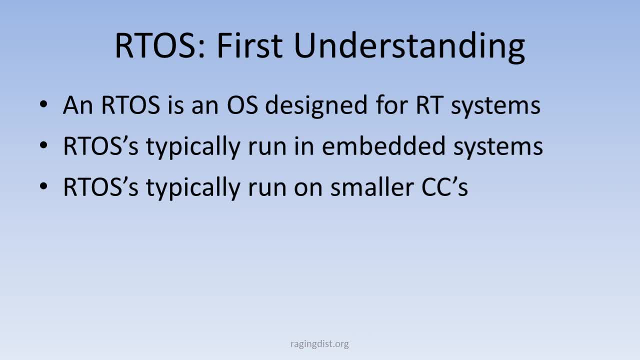 that RTOS that runs in the Aegis system is not an RTOS by the definition of one that runs on a smaller computing complex, because the fire control system in an Aegis, the Aegis RTOS, is just a huge computing complex. So the other definition of an RTOS is one which runs 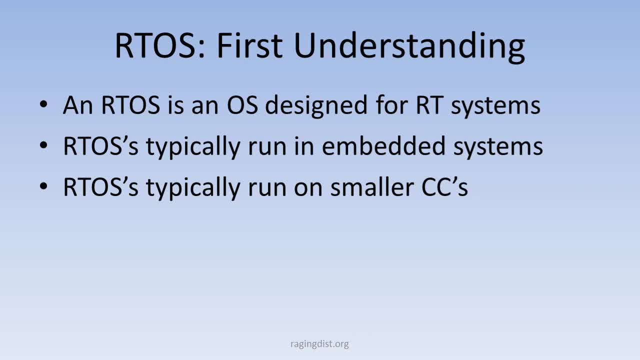 real-time systems on a smaller computing, complex, one that's cheaper, one that fits into a tiny little footprint, say, it's something that runs under the $10 limit. So if you go online and Google the term RTOS and look for a list of them, 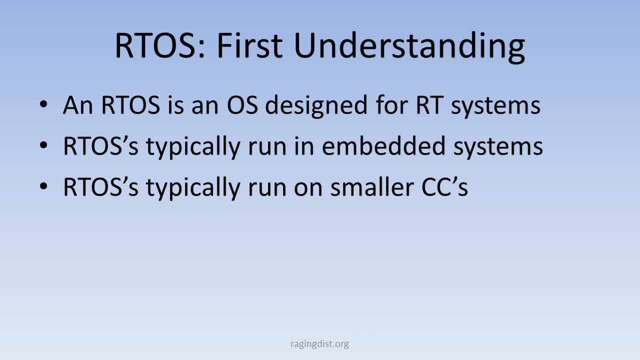 you'll probably find this bottom category for the most part and a few examples from from this, this larger OS thing. I'll continue talking about the specifics of what an RTOS are in another presentation, And come join me for that. There's a lot of things about RTOS I've been doing for years that I'm surprised that people don't know. 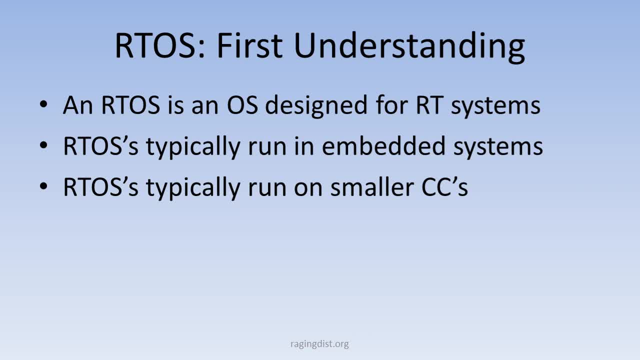 There's not a lot of information out there, And I'll see you then.